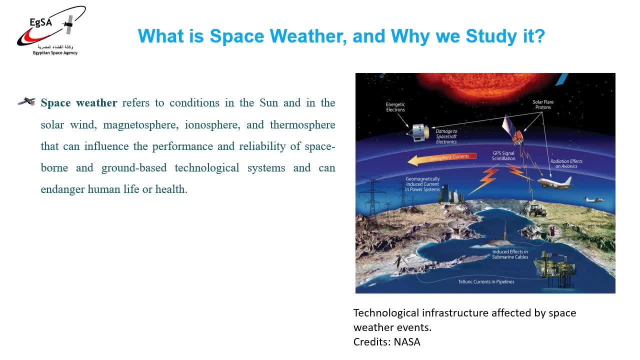 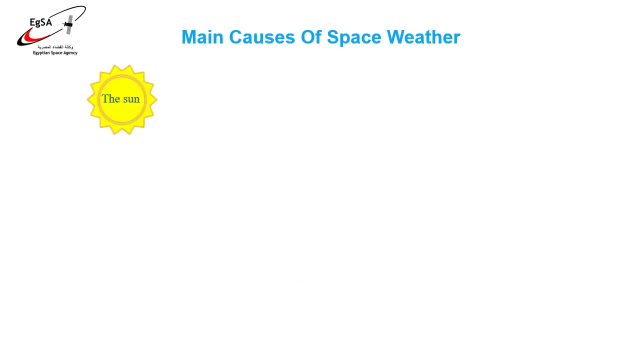 based technological systems and endanger human life or health. similar to earth weather, which can cause damage to homes and other property and disrupt our lives, space weather can cause damage to satellites, create beautiful auroras and affect our communications, navigation and power systems- a matter that can endanger our lives. there are three main factors that influence space weather. the Sun is. 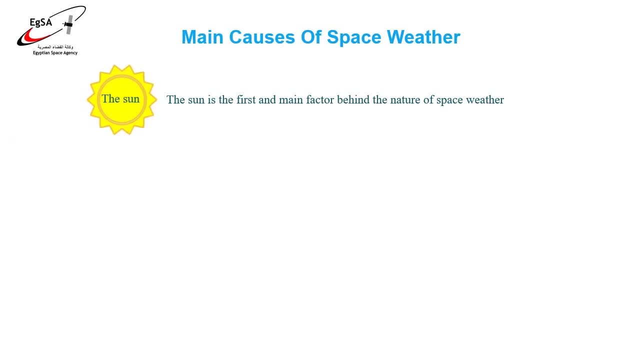 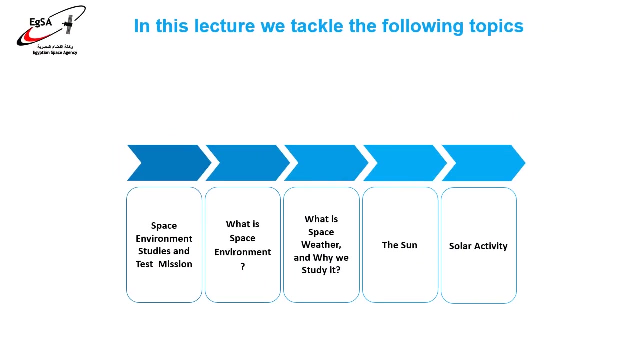 the first, a main factor behind the nature of space weather. so we must understand solar activities such as solar wind, solar flare and CME. the second factor is galactic, galactic cosmic rays. the third factor is meteorites and space debris. the fourth topic is the Sun. 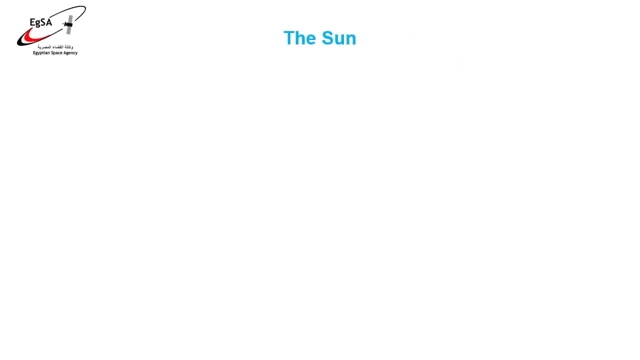 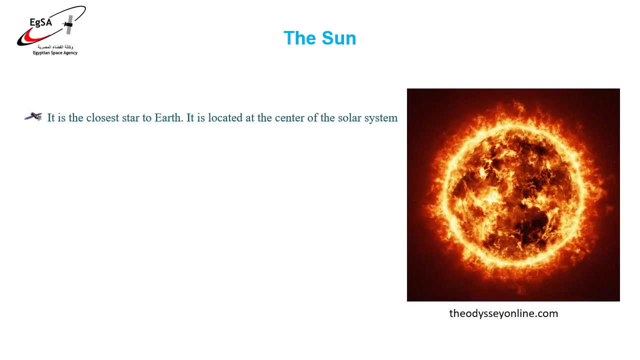 now we get to know more about the nature of the Sun. it is the closest star to Earth. it is located at the center of the solar system. it has the biggest effect on the environment of space. it is a wall of hot plasma about 865 thousand miles away from the sun and it is used to cool down and in the middle of the sun. 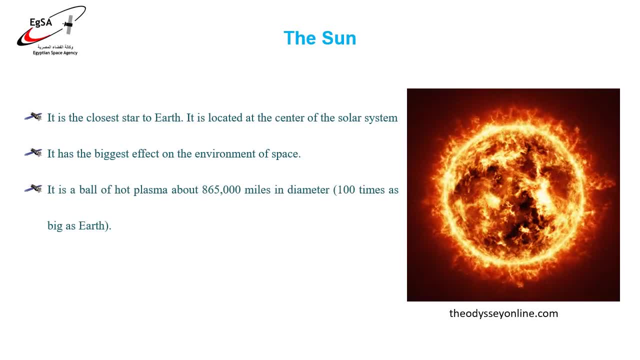 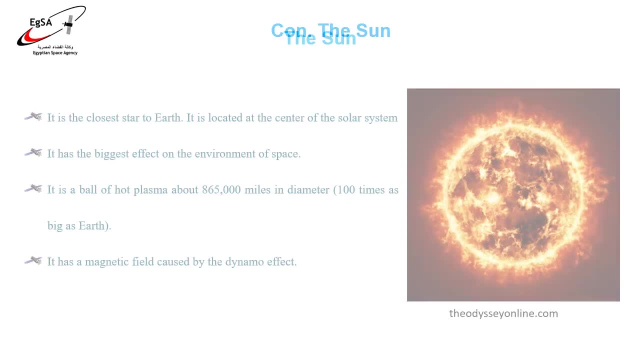 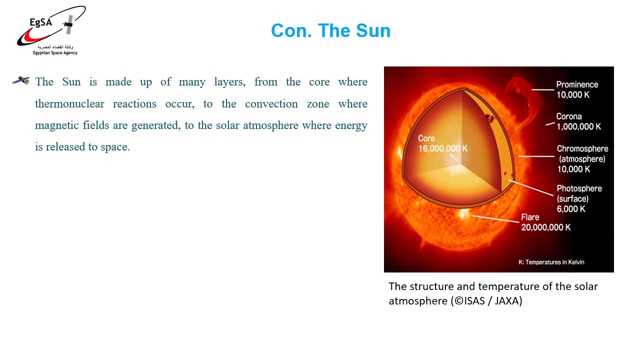 in diameter, which is a hundred times as big as Earth. It has a magnetic field caused by the dynamo effect. The Sun is made up of many layers, from the core, where the thermonuclear reactions occur, to the convection zone, where magnetic fields are generated. to the solar atmosphere, where 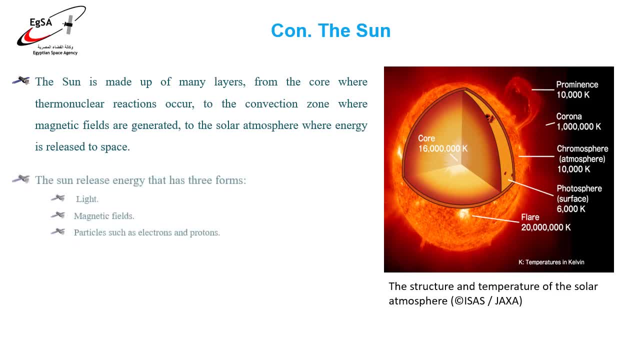 energy is released to space. The Sun releases energy that has three forms: light, magnetic fields, particles such as electrons and protons. Through this energy emission, the Sun releases enormous amounts of material. However, this enormous amount of material is so small when compared to the total mass. 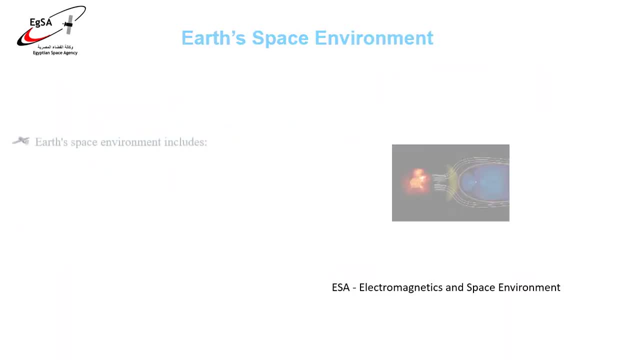 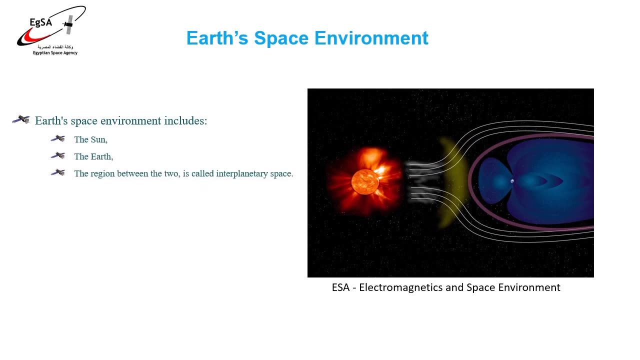 of the Sun. Earth's space environment includes the Sun, the Earth and the Sun itself, Earth, the region between the two, which is called interplanetary space. This environment is filled with plasma and ionized particles, light, magnetic fields. 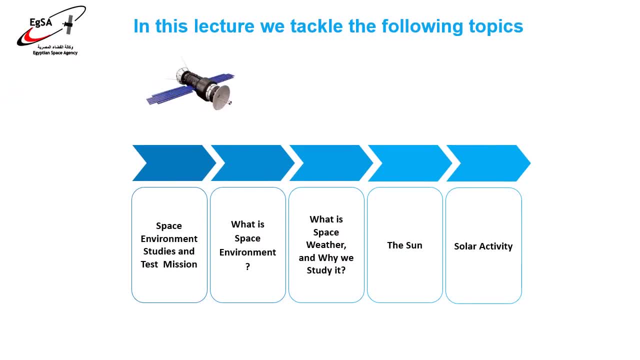 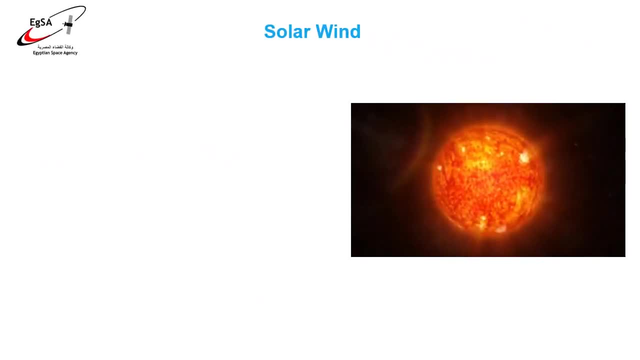 Finally, we move to the last topic, which is solar activity. The first type of solar activity is solar wind. Solar wind is a supersonic flow. Solar wind is the flow of high-speed charged particles continuously blowing off a star, mostly E minus and P positive. 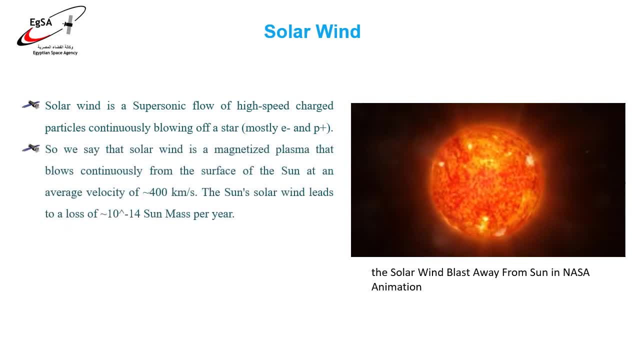 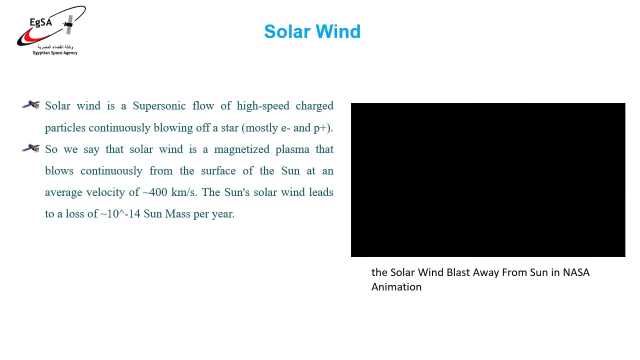 So we say that solar wind is a magnetized plasma that blows continuously from the surface of the Sun at an average velocity of 400 kilometers a second. The Sun's solar wind leads to a loss of 10 to 13 Sun mass per year. 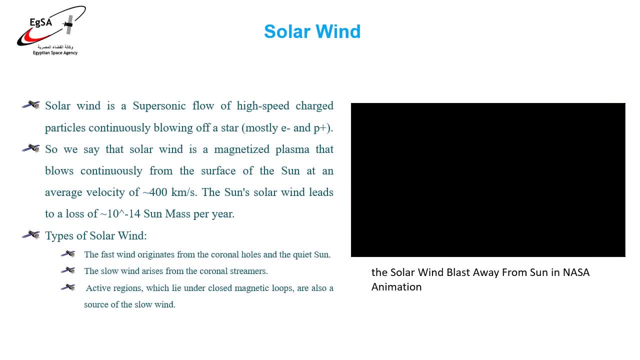 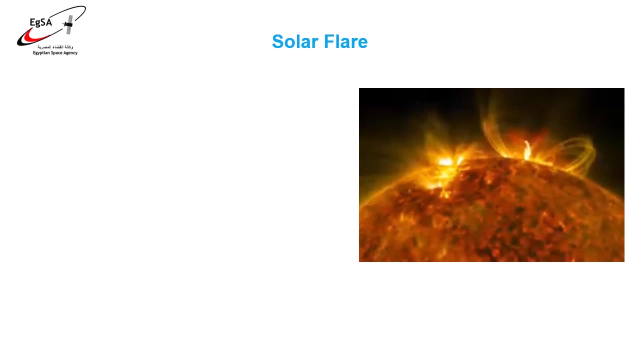 Types of Solar Wind. The fast wind originates from the coronal holes and the quiet Sun. The slow wind arises from the coronal streamers. Active regions which lie under closed magnetic loops are also a source of the slow wind. The second type of solar activity is solar flare. 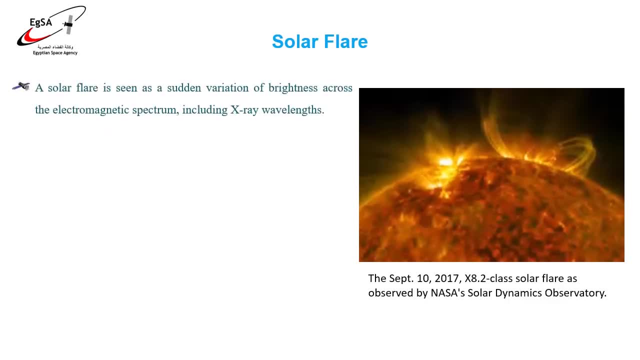 A solar flare is seen as a sudden variation of brightness across the electromagnetic spectrum, including X-ray wavelengths. This often leads to the acceleration of electrons and protons traveling to Earth at near relativistic velocities- in excess of half the speed of light. The X-rays reach Earth and ionize some of the upper atmosphere in only 8 minutes without 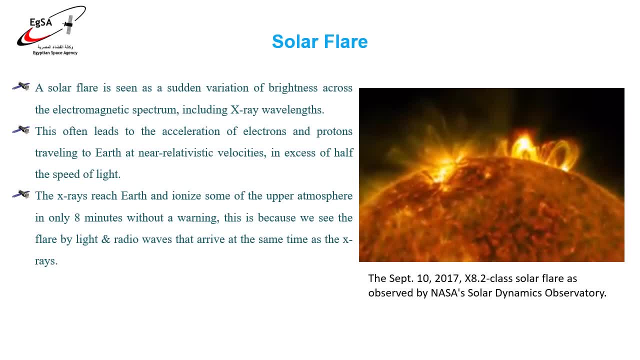 a warning. This is because we see the flare by light and radio waves that arrive at the same time as the X-rays. At these speeds, protons can reach Earth in around 15 minutes. The second type of solar wind is the slow wind. 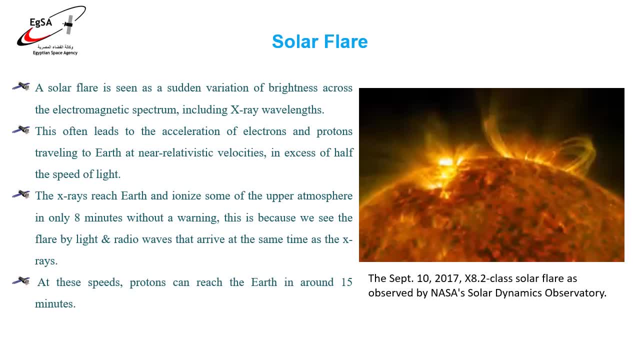 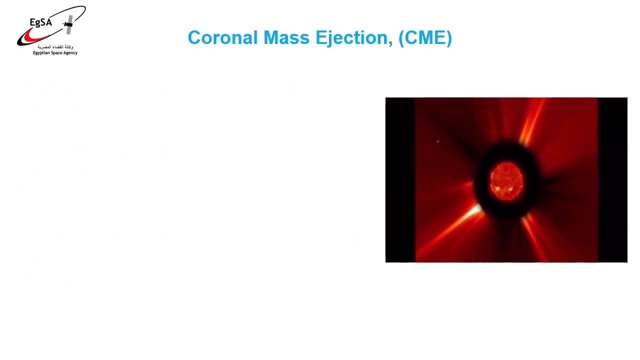 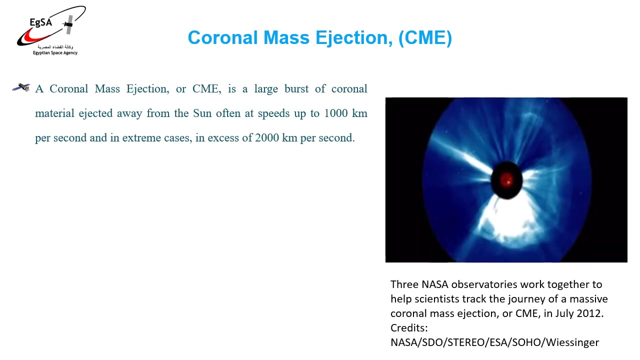 The fast wind is seen as a sudden variation of the solar flare. This often leads to the acceleration of electrons and protons traveling to Earth in near relativistic velocities, in just about half the speed of light per second. The slow wind is seen as a sudden variation of light and radio waves that arrive at the 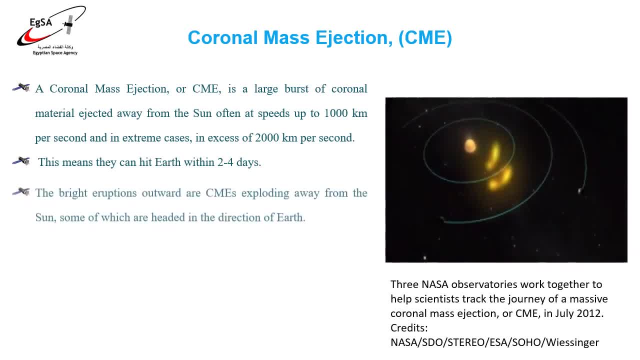 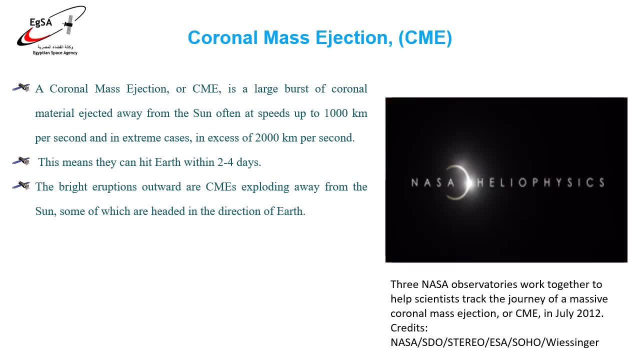 in 2 to 4 days. The bright eruptions outward are CMEs exploding away from the Sun, some of which are headed in the direction of Earth. The extra plasma load can stretch the magnetosphere back out, away from the Sun, and when the magnetic